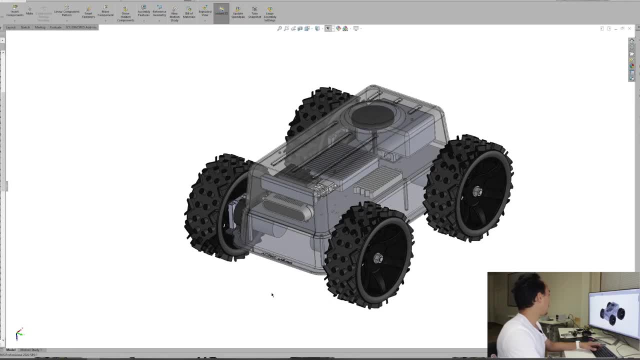 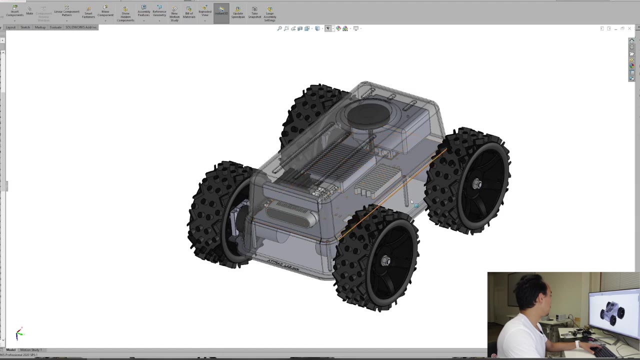 here Let's get started. Okay, here we are. This is the CAD model of the Adler, So I will explain and do the hardware overview on here, which is quite easier to see things. So the Adler body is just only the two carbon plates which connect together with these simple aluminum pillars. 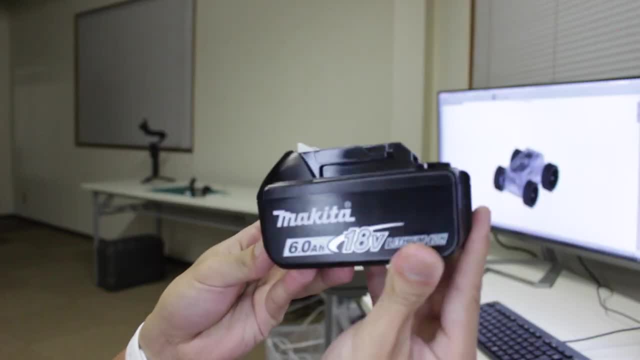 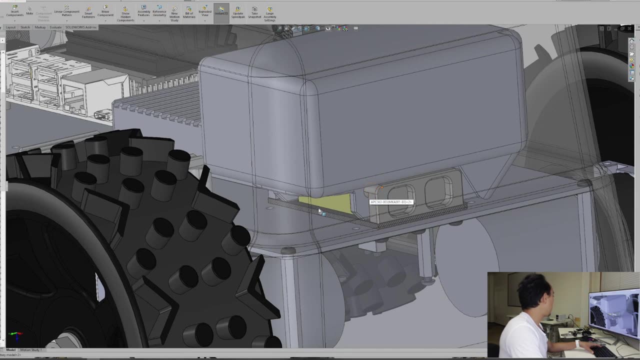 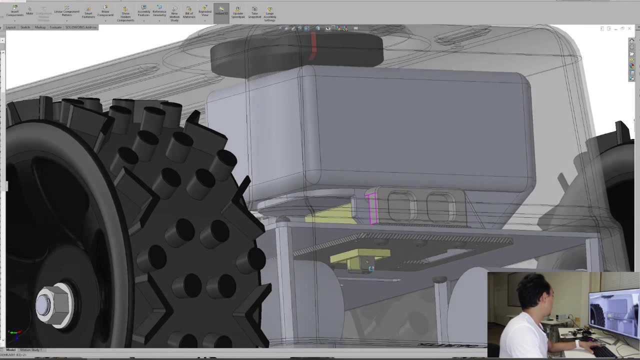 So at the back of the Adler- here you will see this is the Magita battery 18V 6A And we designed this aluminum parts to hold the battery together And there is a simple carbon plate up and down to let everything fix together in the body. 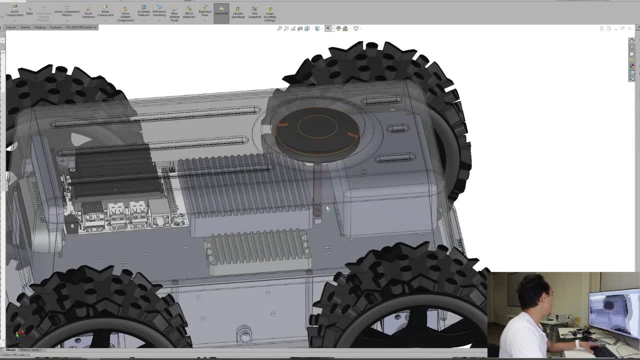 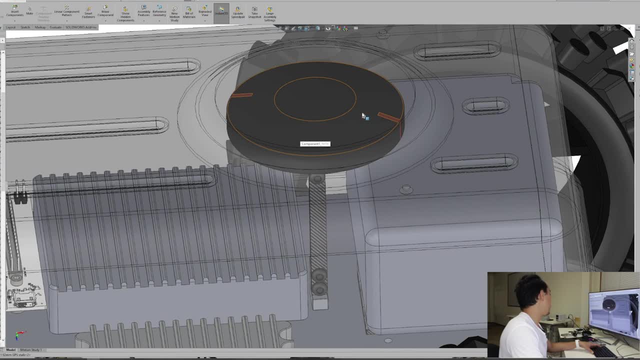 And next to the battery. this is the GPS pole, and we are using HEAR 3 GPS, but of course, if you have the HEAR 2 or HEAR Plus, you can use it as well. And next to the GPS pole is the battery. 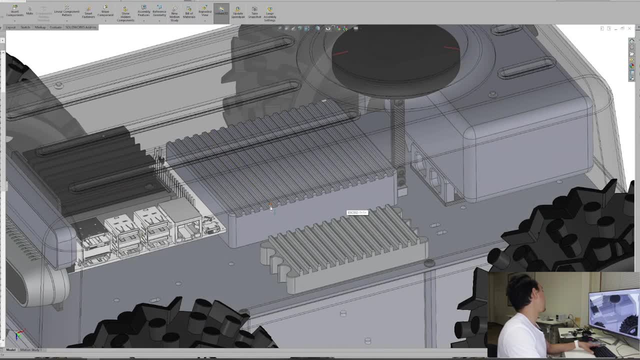 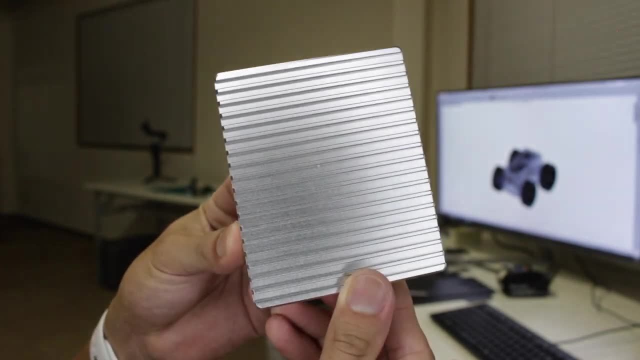 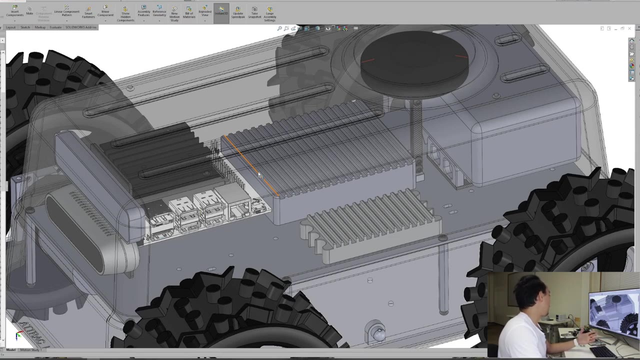 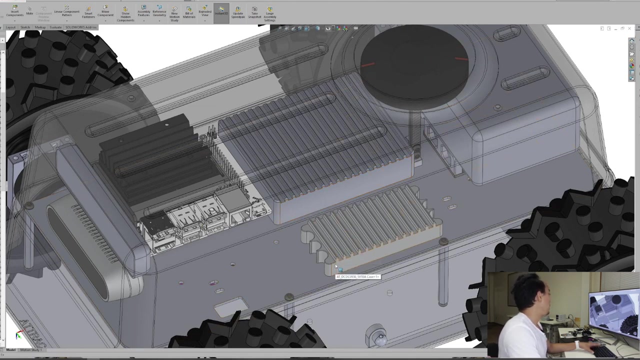 This is the 2-channel ESC motor driver which gonna drive the left side and right side motor. So basically we just use the 2-channel of the PWM input from the Adupilot or any receiver to drive the motors Next to the ESC. you will see, this is the 5V, 10A DC-DC regulator for the Jetson Nano. 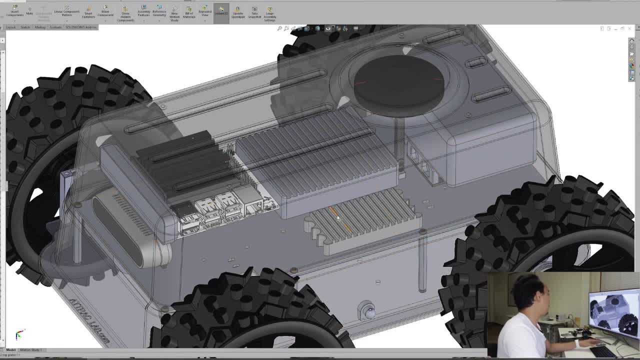 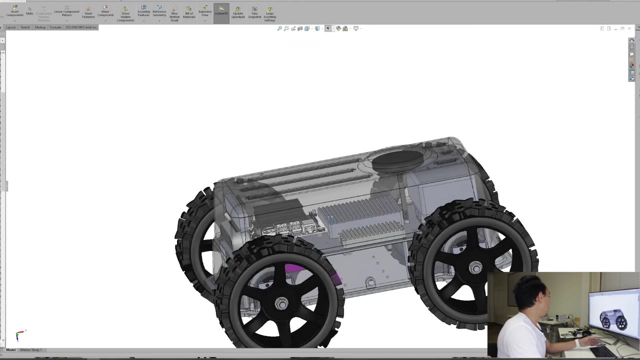 So in case, if you don't wanna use the Jetson Nano, but you wanna use something like the Savia NX or the Intel NUC, you can change this regulator to 12V or 19V, just depends on what you want. So in front here there is the 2 cameras. 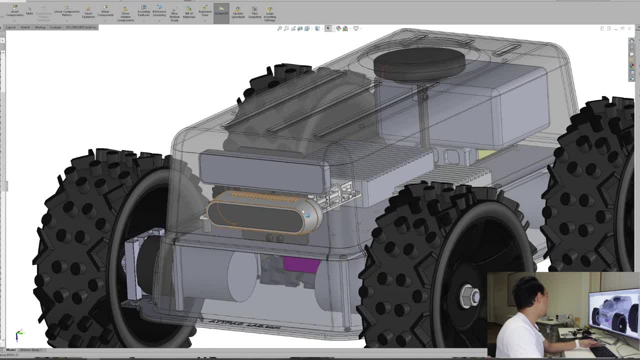 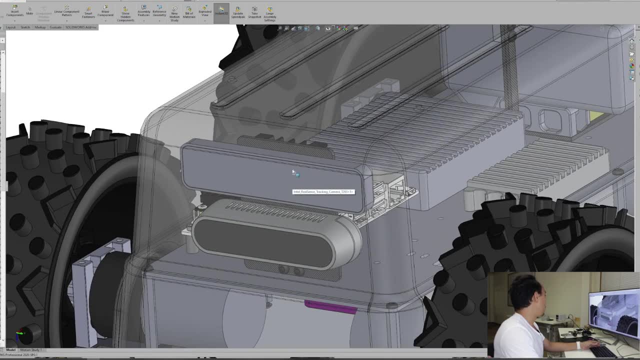 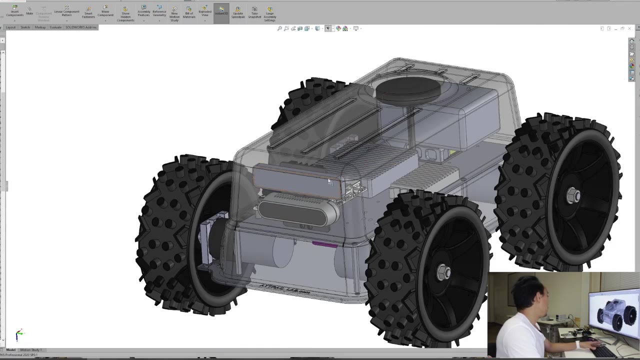 One is the D435 Intel RealSense, which gonna give us the distance information, And the upper here, Which is the T265, which can provide the odometry information. So in case we wanna run the robot indoor and we cannot get the GPS information. 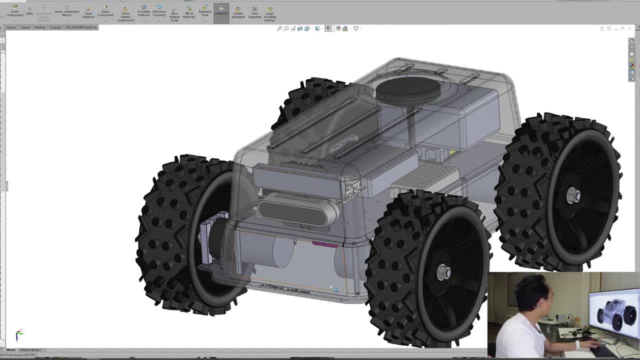 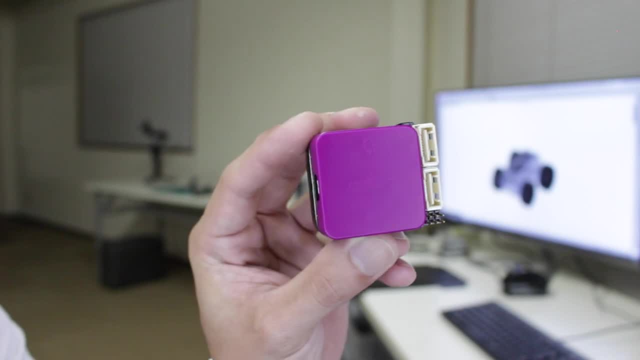 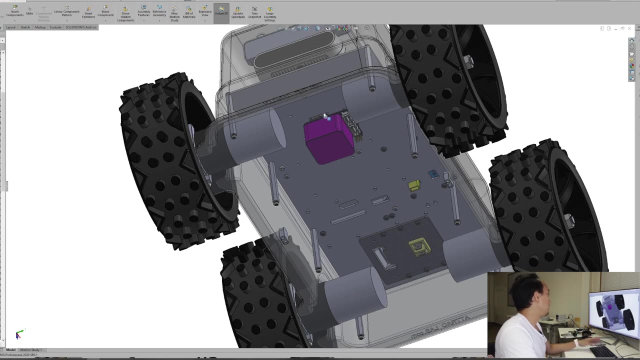 So the T265 is the way to go. So under here this is the Cube Mini Purple which running on Adupilot software. So if you're interest in the autonomous drive vehicles and the open source project, this is the way you should go. 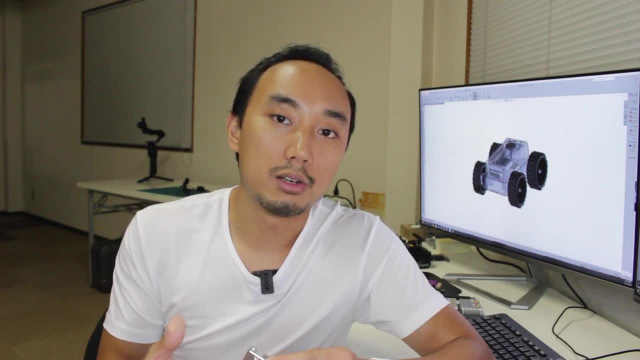 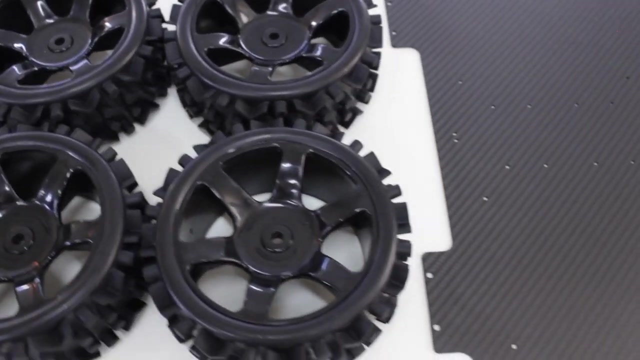 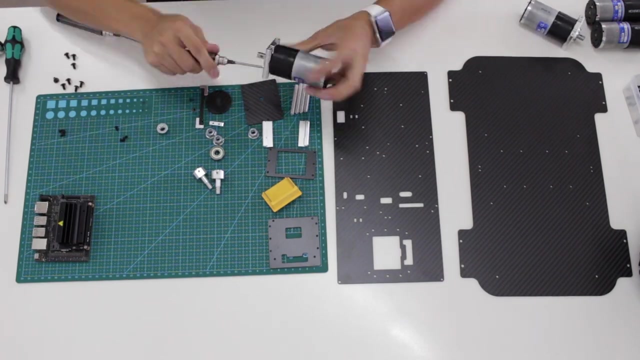 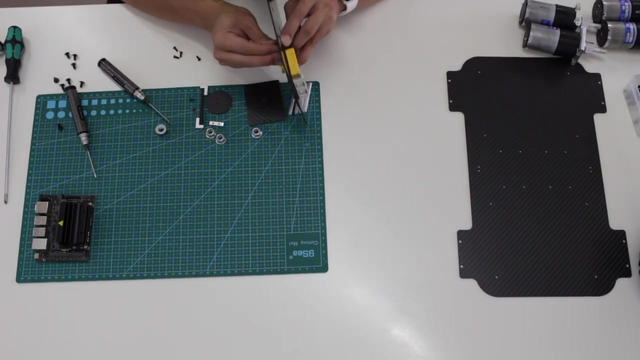 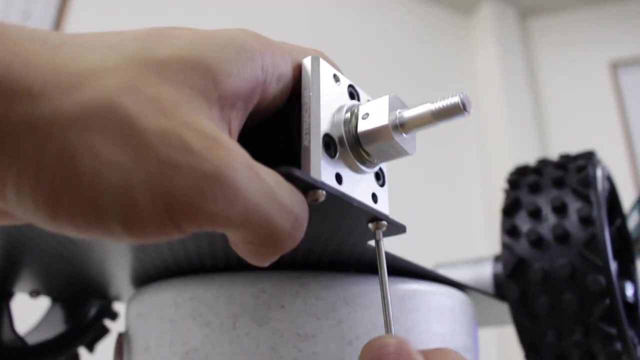 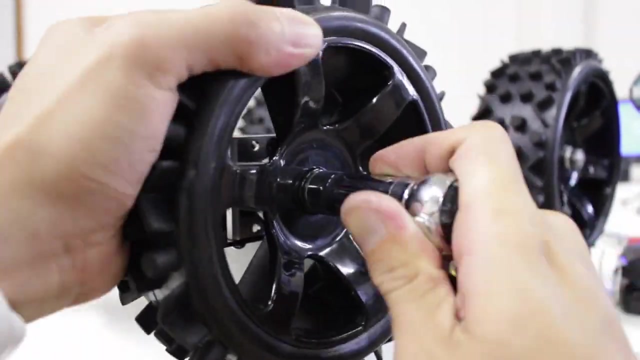 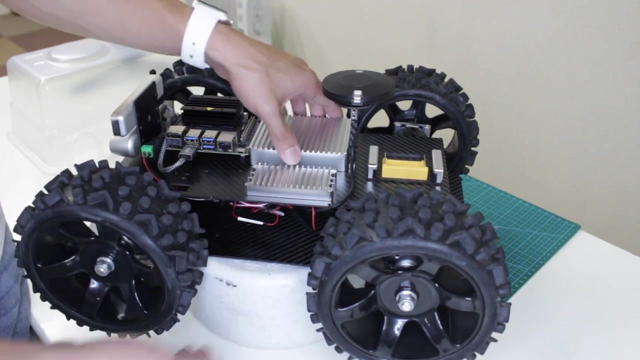 And next I will show you how to assemble the outlets from scratch And do some tuning in the mission planners And at the end it will be some demonstration. And here we are. This is the Adler after finish assembly. But I still need to connect the motors to this ESC port. 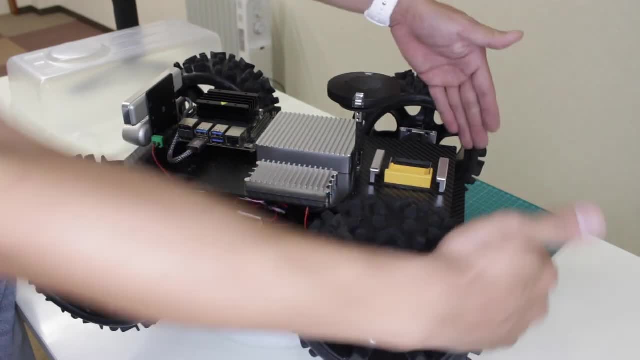 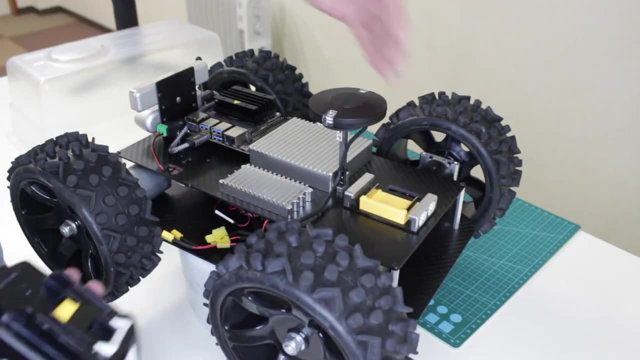 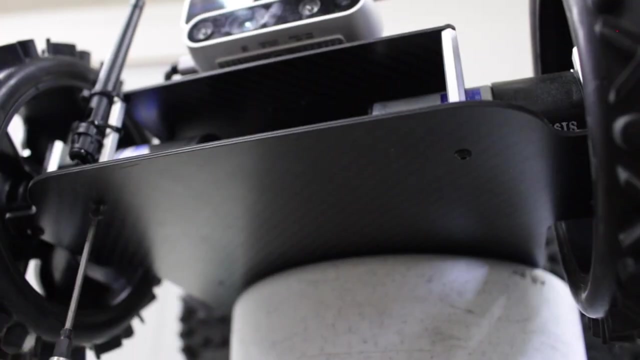 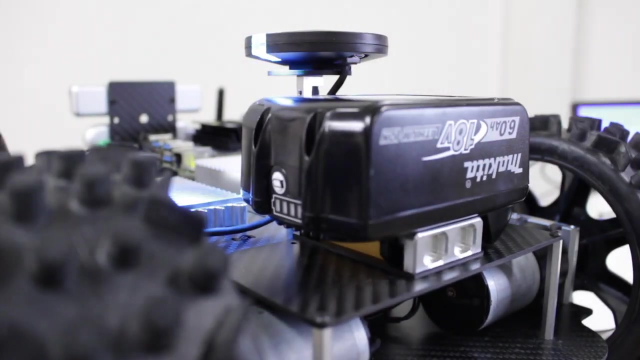 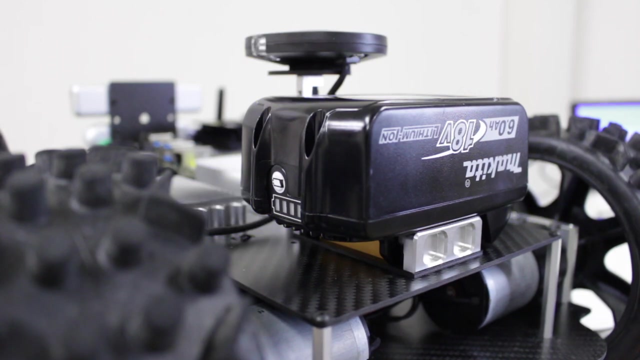 And then I will tie this 4 screws to connect the upper plate and the bottom plate together, And after we connect the battery to the battery holders, it will ready to go. Okay, now I'm connecting the Adler to my laptop And open up the mission planner. 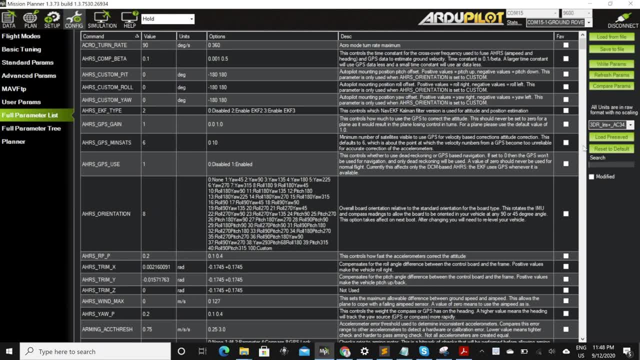 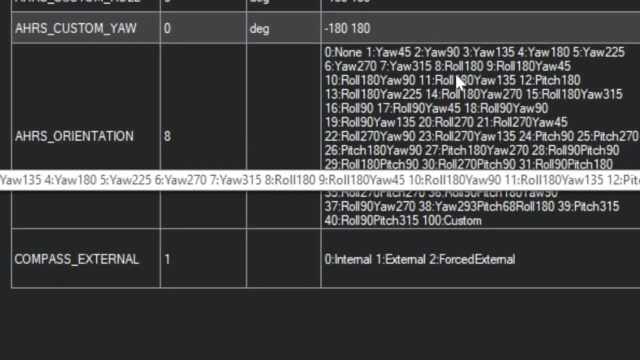 So first we go to the config page And click on full parameter list. The first parameter that we need to set is AHRS orientation To set the correct orientation of the Cube Mini that placed on the Adler. So it was set as 8 for roll, 180 degrees. 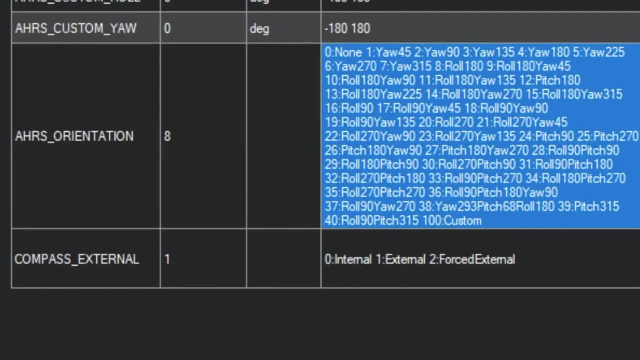 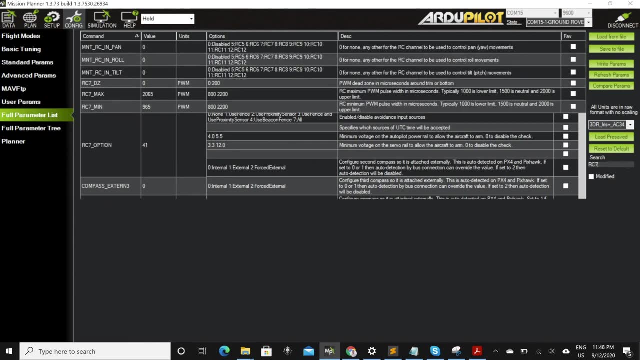 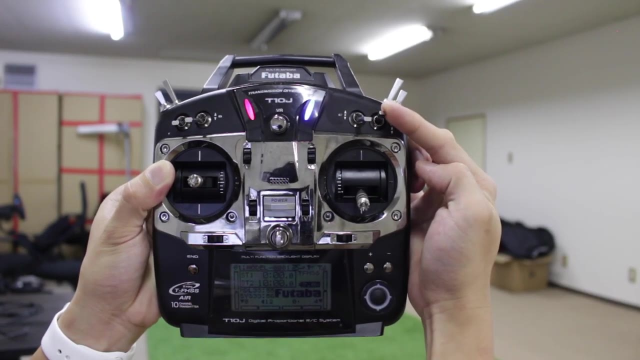 So if you want another orientation, you can change it as well. So the next parameter is RC7 option, Which is for arm and disarm. So it depends on which transmitter you are using. So in my case I'm quite get used to with this channel. 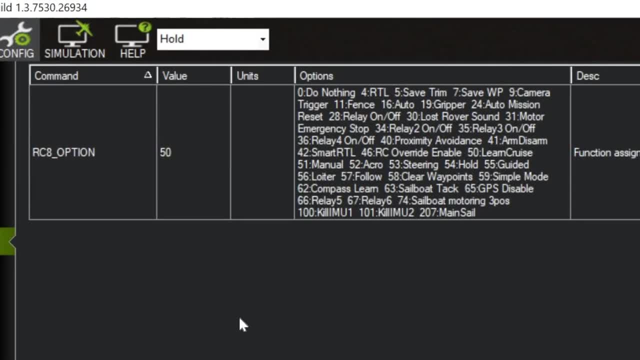 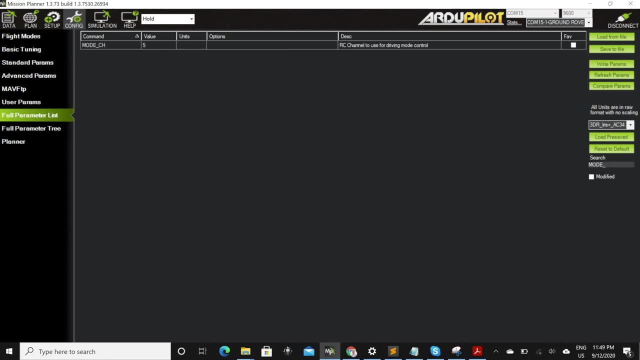 So the next parameter is the RC8 option for learn cruise. So when we are tuning this throttle speed controller, it will be useful for us. So we just set it as right now. So next parameter is the mode CH, Which I set it as 5.. 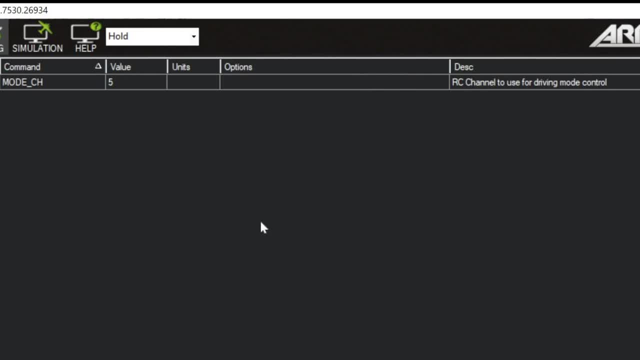 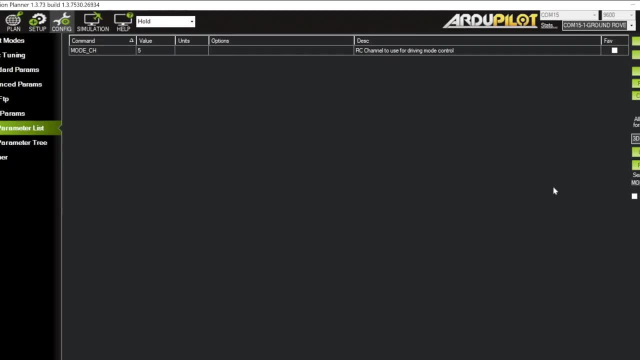 So on my transmitter on the channel 5, it is 3-way switch So I can use the whole and manual and auto mode in this switch. So if you have another switch that you want to use, you can set it as well. 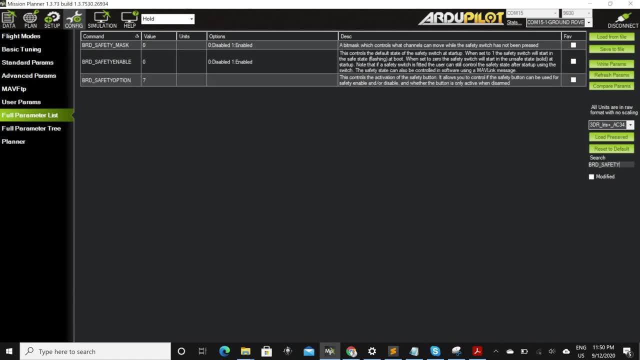 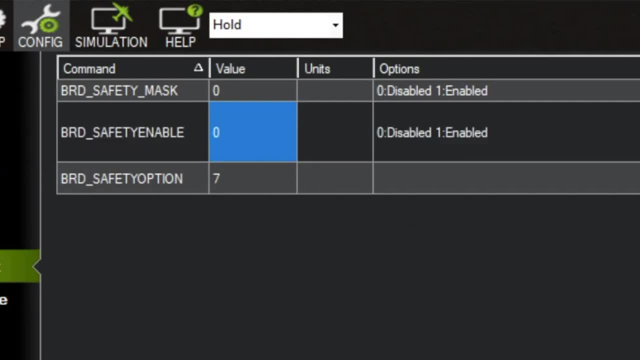 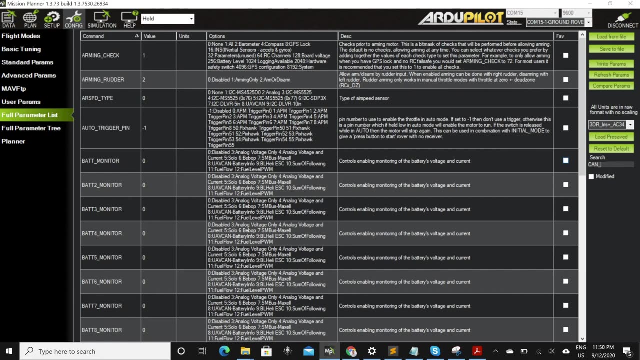 So next parameter is BRD, Which is the safety enable. In our case. our GPS doesn't have the safety switch button, So we just disable it here. So next parameter is related to our GPS, Because we are using here 3.. 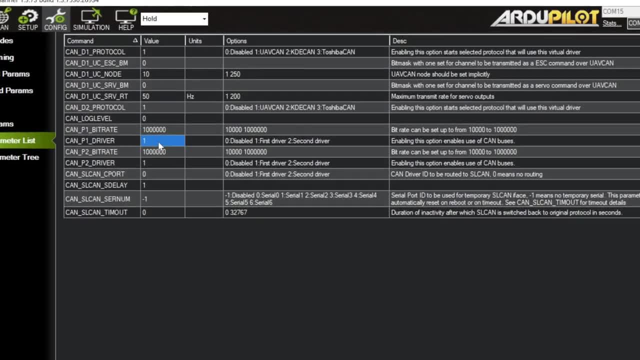 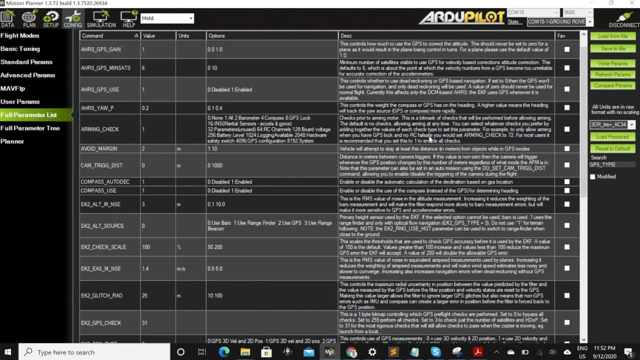 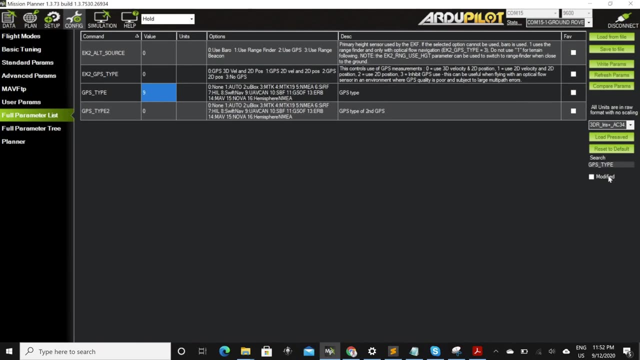 And it support the UAV CAN. So we need to set CAN D1 protocol and CAN P1 driver as 1.. So next it is GPS type. We set it as 9 for the UAV CAN And the last one is the NTF LED types. 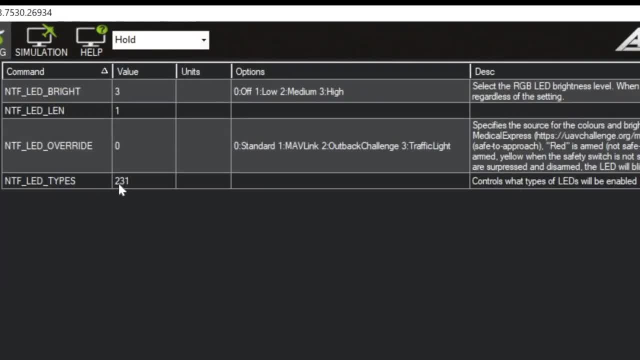 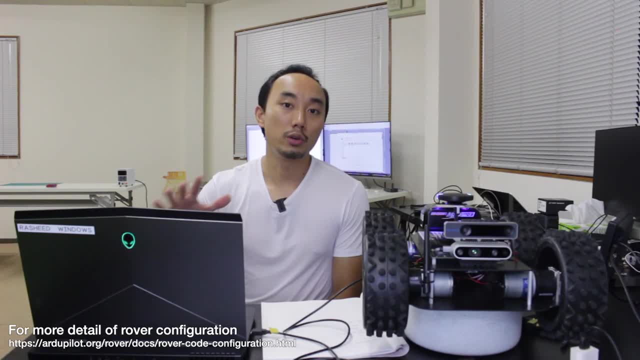 For the LED indicator, we set it as 231.. So that is the basic parameters that we need to set before doing everything Like calibration and tuning. So next we need to do the mandatory hardware checkup, Like accelerometer calibration, Compass The radios. 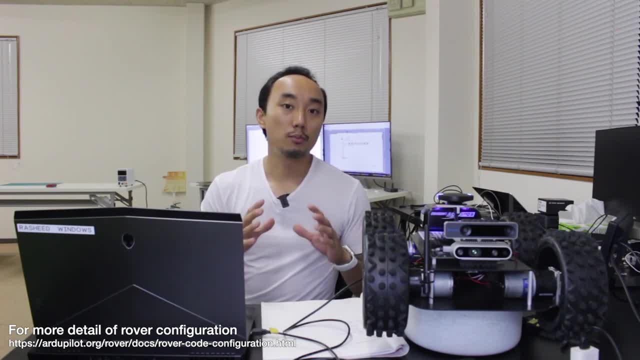 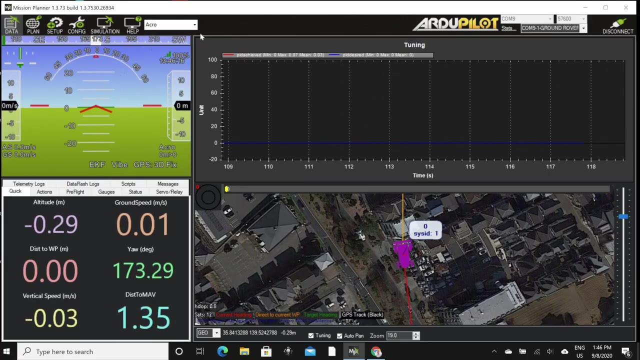 The servos To check that everything working properly. But I already done that, So next I will do the tuning. So let's see how I tune this guys For the throttle and steering, And next we will do the waypoint demonstration. So this is the most time consuming process. 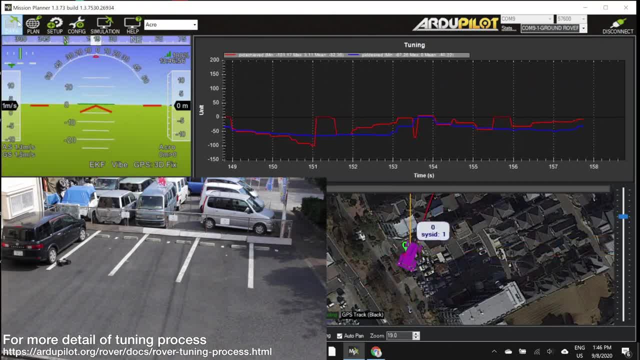 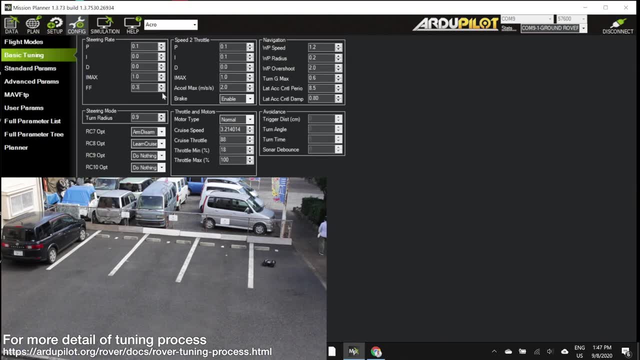 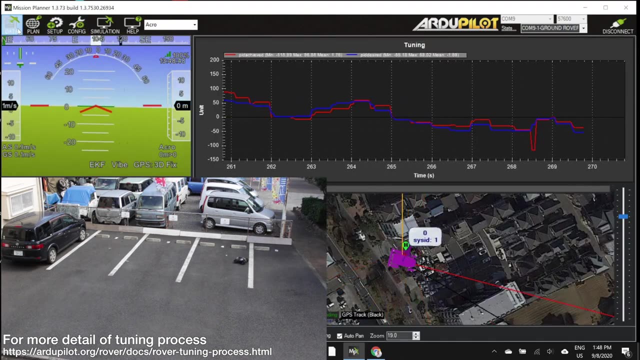 So first we need to tune the throttle speed controller. If you remember that, I set RC8 option as learn cruise, Which allow the rover to get speed data and matching it with the input throttle. And please remember that the cruise learning process should be done in manual mode. 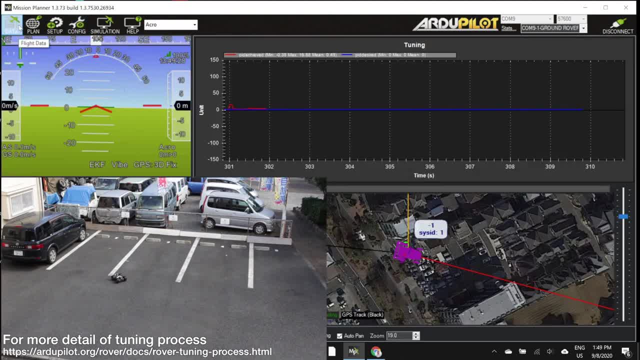 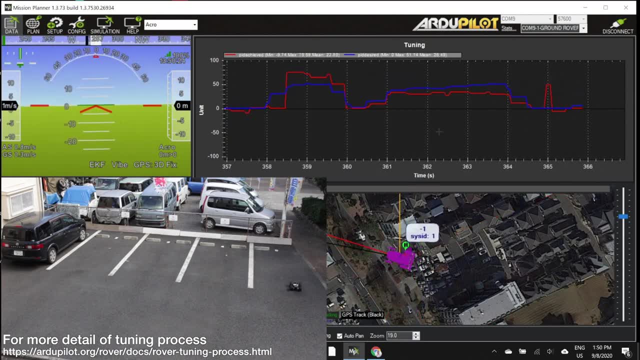 So after we got the baseline from cruise learning, We need to set parameter GCS PID marks as throttle or steering Depends. on which do you want to tune? And on the data page. we need to open up tuning graph window. Then check the box of PID design. 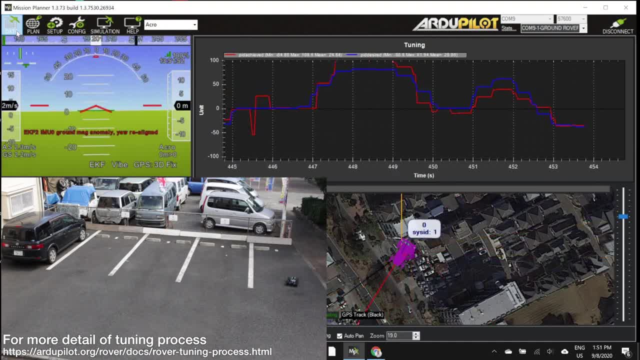 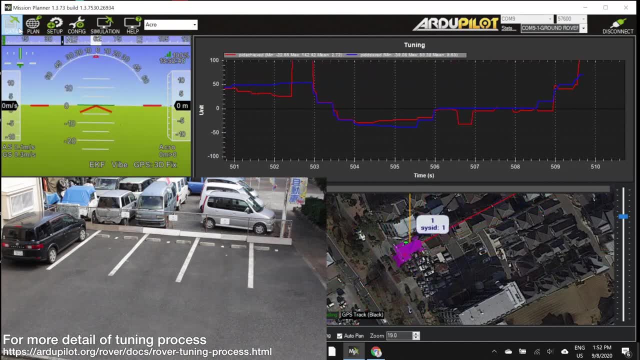 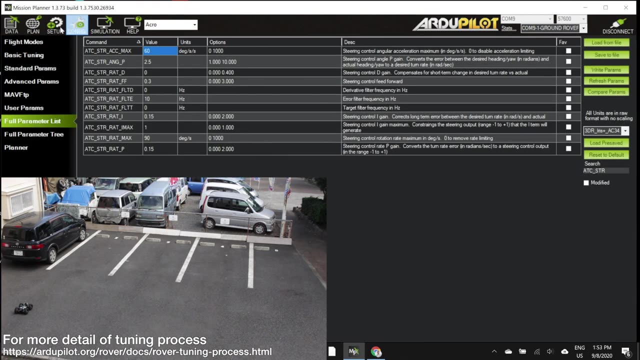 And PID achieve. From now we will use acro mode to tune the PID of throttle and steering. So, as you may know, PID tuning is kind of trial and error process. So you can try, change the value of P and I, And mostly we keep D as default. 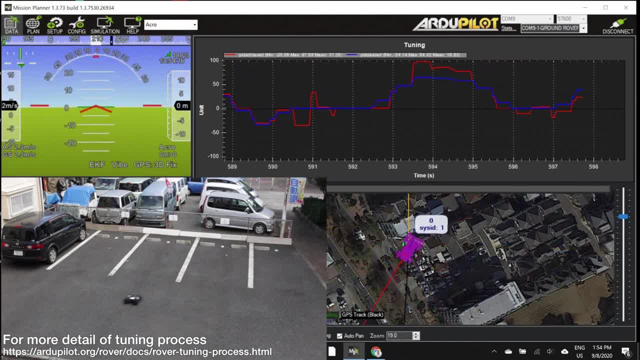 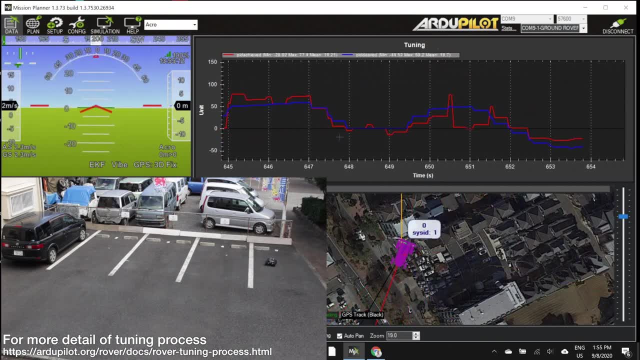 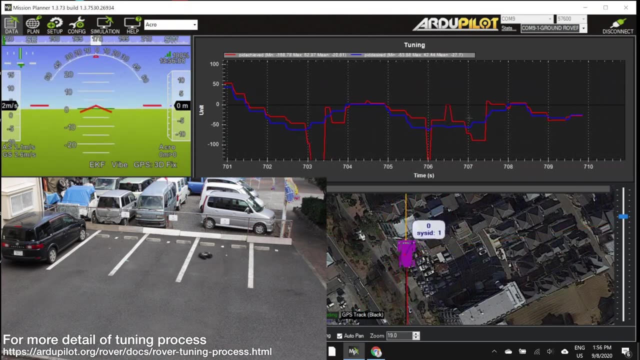 For steering rate tuning You should start with feed forward or FF value. So this is also kind of baseline for steering. After that You just adjust the P and I to make it reacts as you want. So I highly recommend you to go check on Adupilot documentation page. 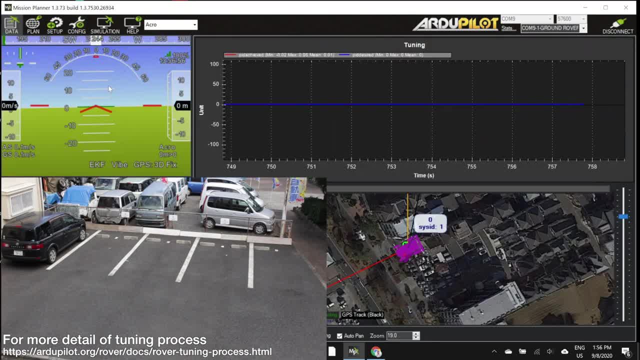 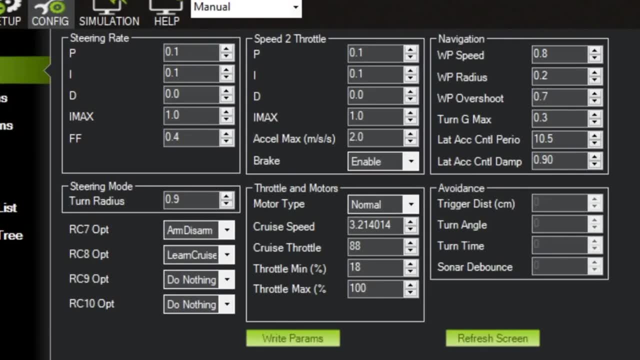 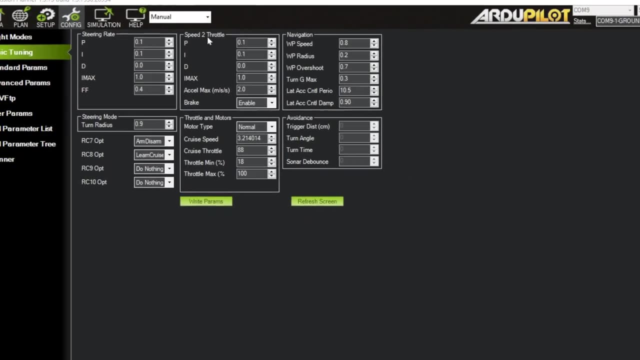 Because that is the best way you can follow it step by step And it was explained very well. And these are the final values of the PID steering and throttle From my tuning process, So I think it's pretty much ready to go test autonomous drive right now. 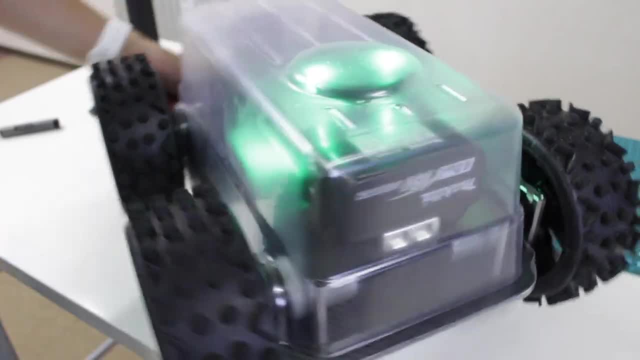 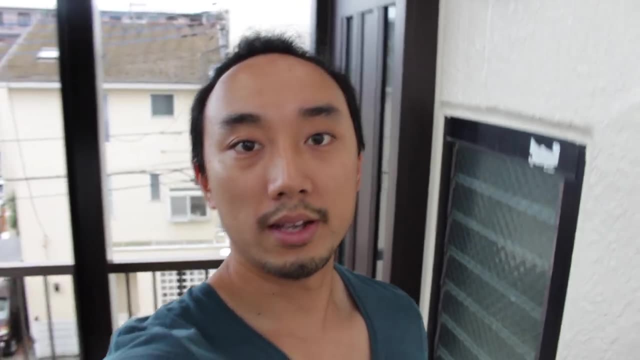 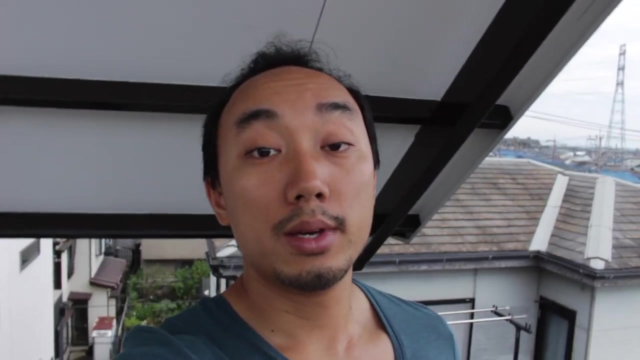 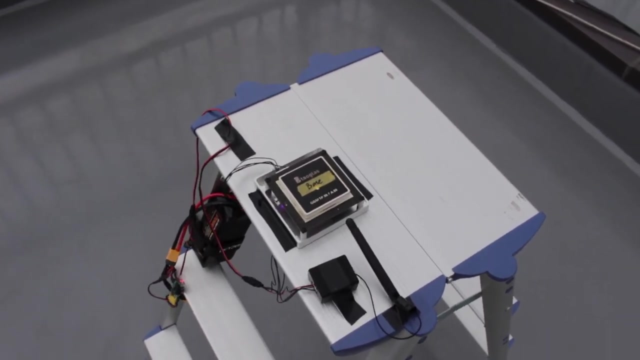 Ok guys. So before we test the waypoint, I would like to show you something. I would like to set up the base station to use the RTK GPS. So here I'm, at the roof of my company building. So this is just a simple base station that I can do for just a test. 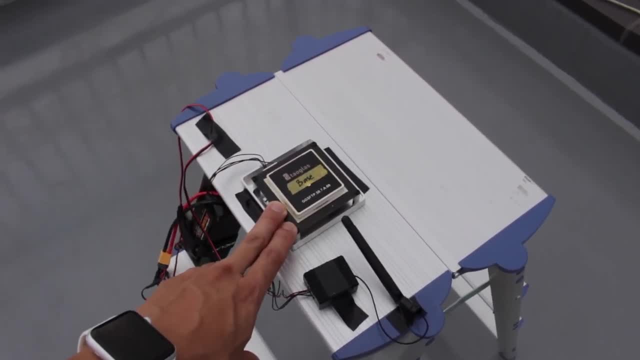 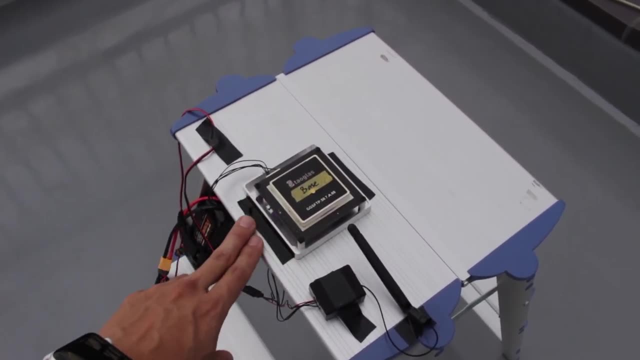 So this is the F9P GPS, So you can find it in the internet. It has many resources about how to set up the base station for the F9P, So it will just give the data from this UART port, The UART2.. 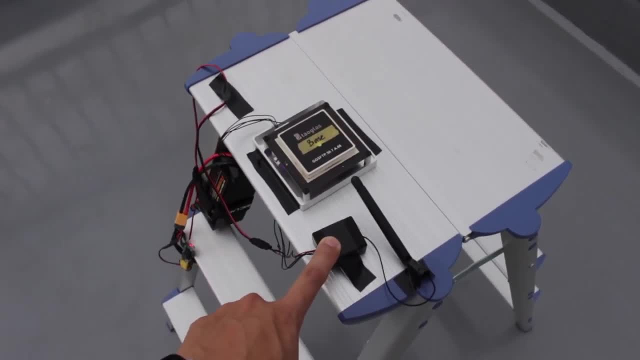 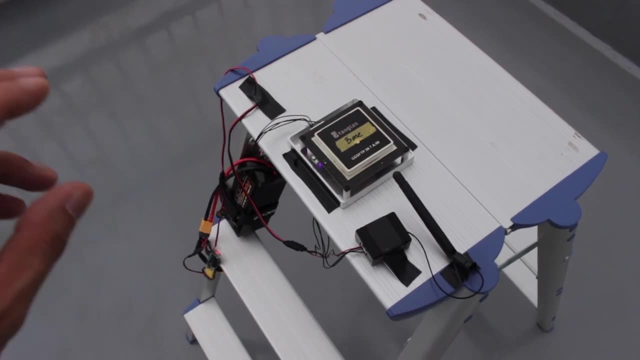 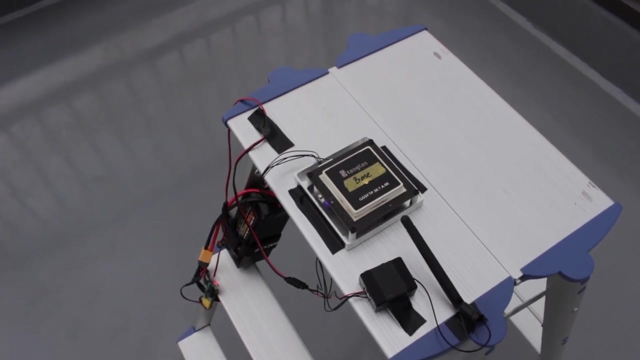 And it will goes into the XB And I have another XB on my desktop And that XB will just inject the RTK RTCM correction into the mission planner And we can get more accurate result for the position. Ok, I'm come back to the first floor again. 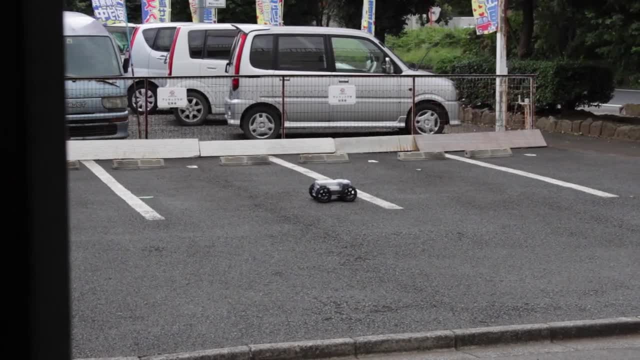 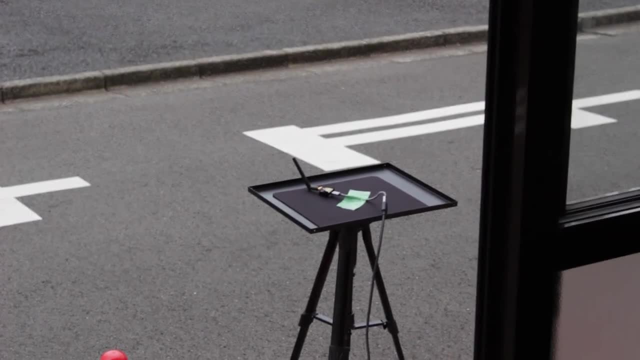 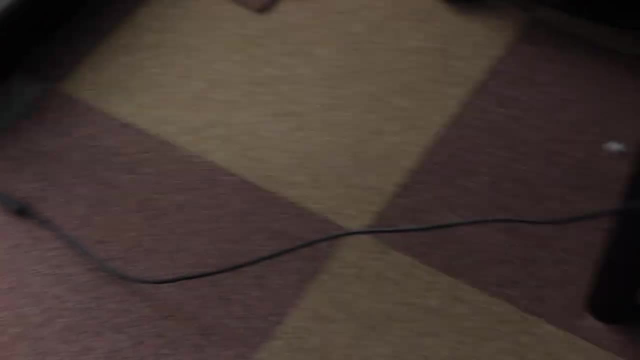 And the Adler is waiting for me outside, Ready to do some demonstration. And here you can see another XB that received the RTCM correction from the base station GPS And it just connect to this long USB cable And it connect to my laptop here. 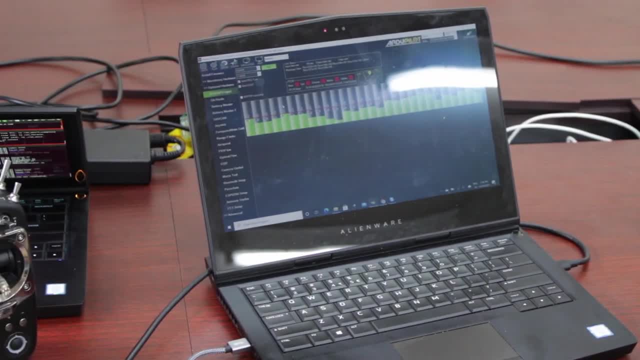 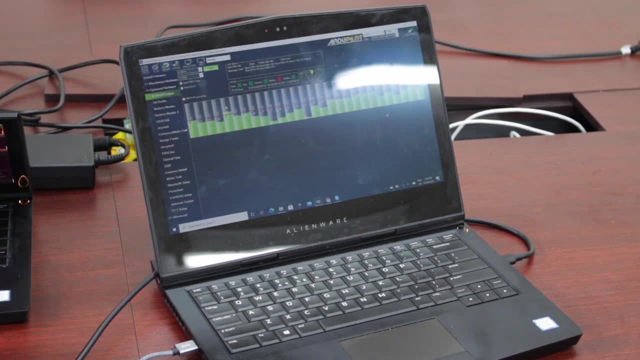 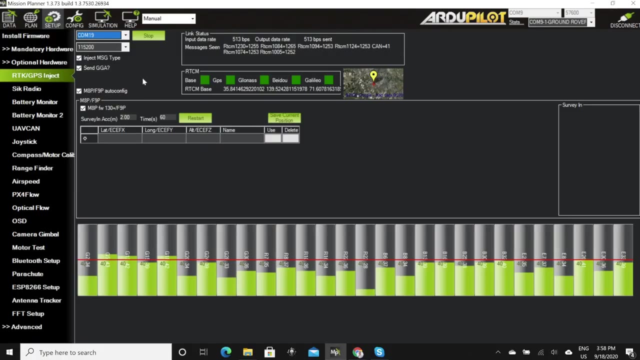 Which is open up the mission planner. So it will just inject the RTCM correction to the mission planner And we can get more accurate result to control the robot. On the optional hardware menu, RTK GPS inject, You will see I'm connecting to COM19 port to get the RTCM correction message from my GPS base station. 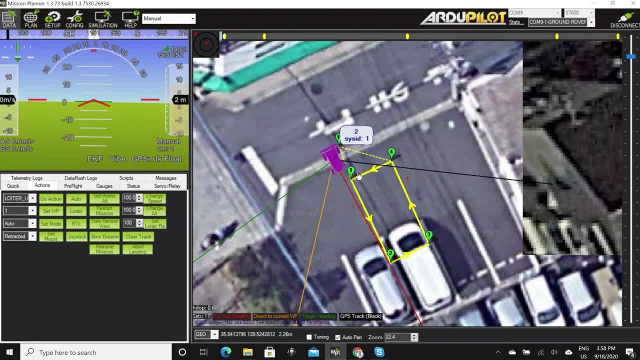 And on the data page my GPS status is showing RTK float, Which means we can get an accuracy around 10 to 20 centimeter, Which sometime is jumping around on the points, as you can see. So I did some simple experiment that if the GPS position is higher, like 1 or 2 meter from the ground, 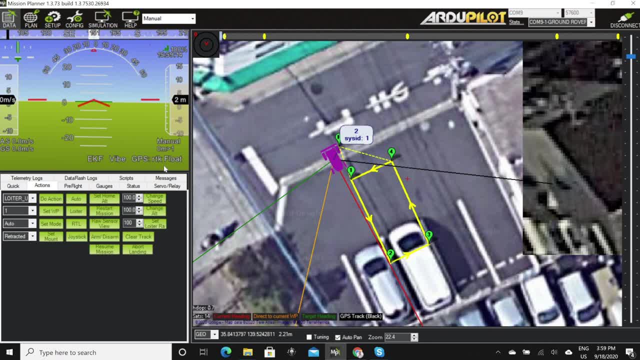 We can get easily the RTK fix, which mean 1 centimeter accuracy. But anyway, this is not that bad for the small size robot And we can still do a demonstration. So I'm making a simple waypoint, like this small rectangle course. 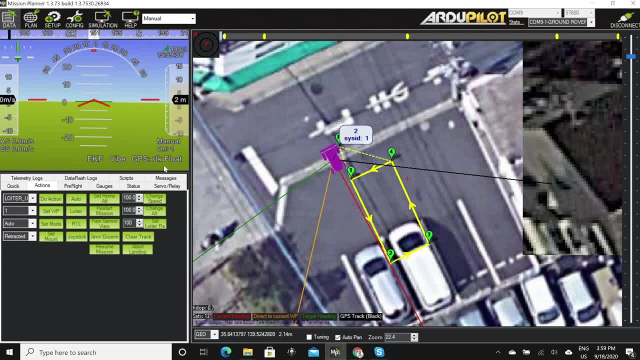 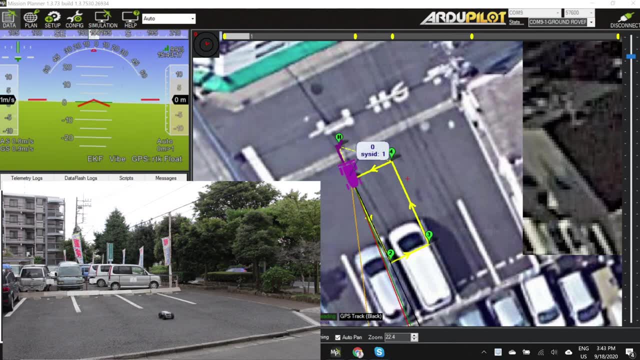 And I will switch to auto mode And it will just run by himself. You can see it's a little bit weaving and still some overshoot, But it can go in straight line and stop at the point. So we can try tuning it up a little bit to get a better performance. 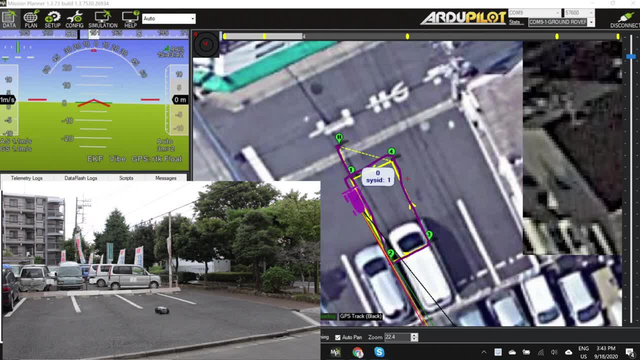 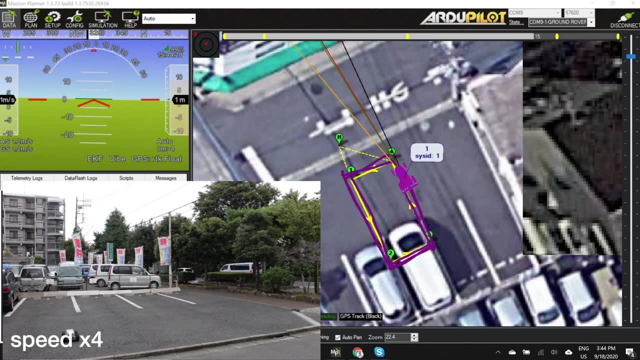 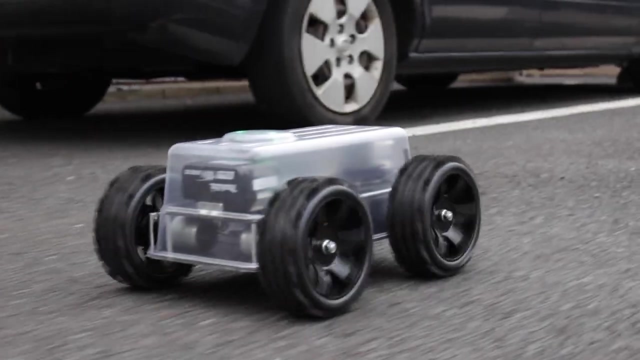 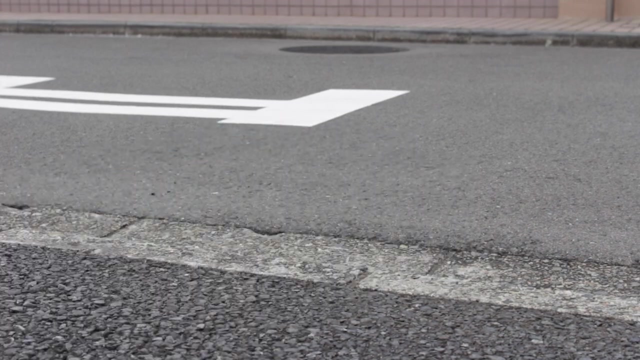 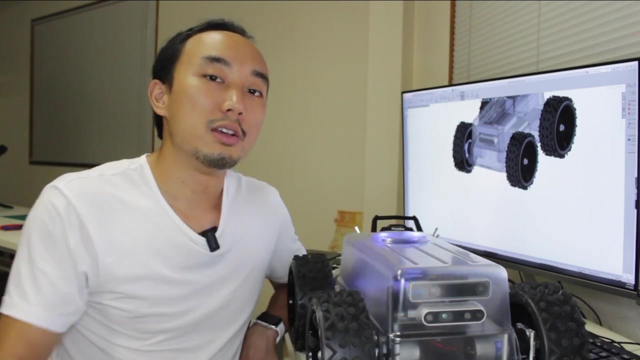 But it's pretty much depends on which kind of application you want to apply to. But I think this is quite enough for just a demonstration And that is the overview of the Atlas and some basic operation that this guy can do. So next I would like to do something more interesting, like some object detection and object avoidance. 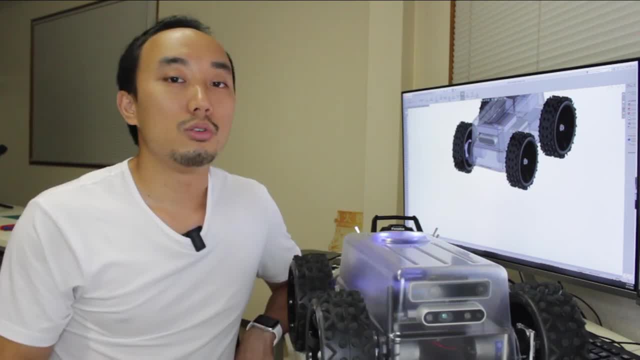 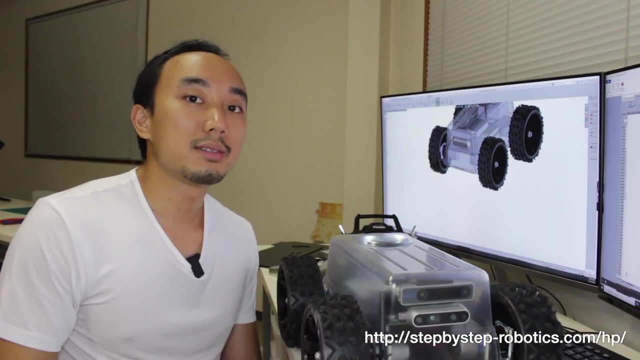 And doing a slam by using the LiDAR. So there are a lot of things that I want to do with this guy. If you're interested in the Atlas, please go check out on my website, stepbystep-roboticscom. 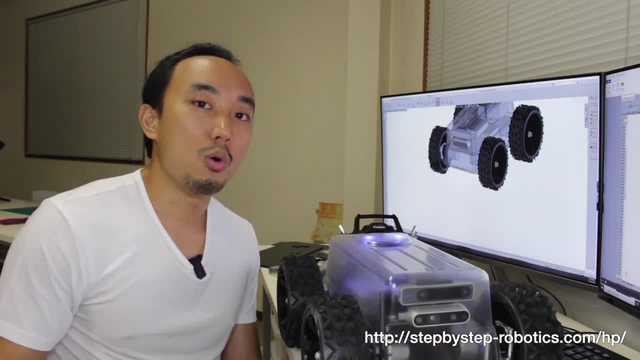 So please stay tuned And thank you for watching.